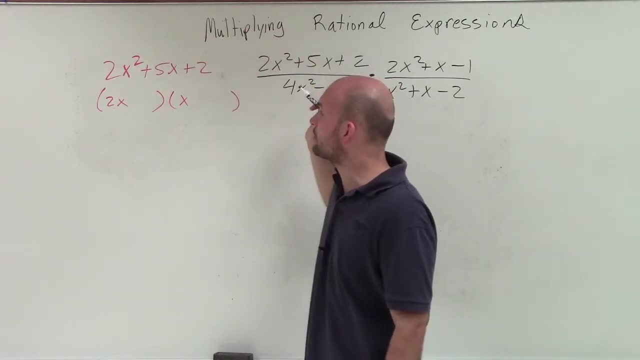 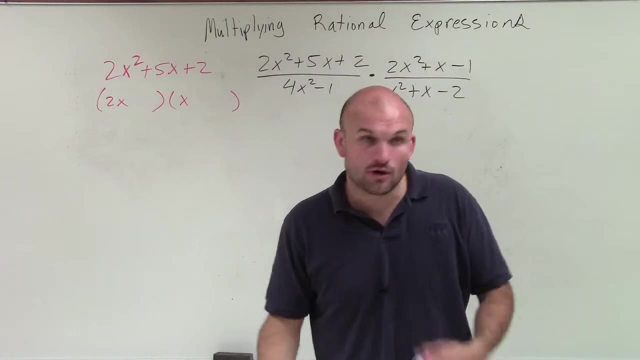 or at least without dealing with our fractions that we're going to deal with, then what we're going to do is say, all right, the last two terms have to give us 2.. So our only options there are positive 2 and positive 1, or negative 2 and negative 1.. However, the terms have 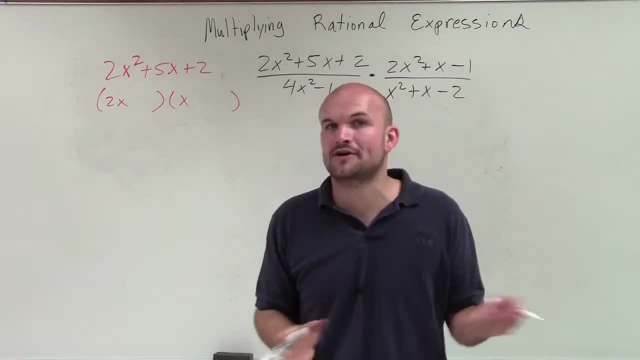 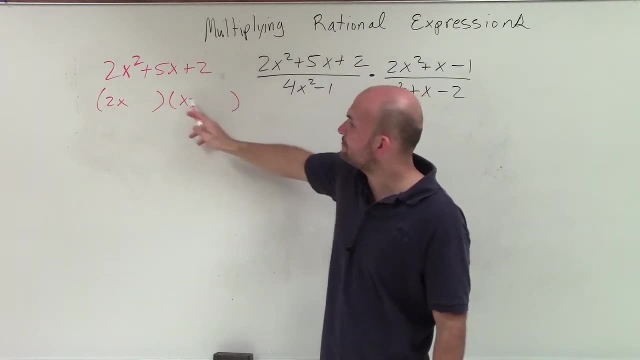 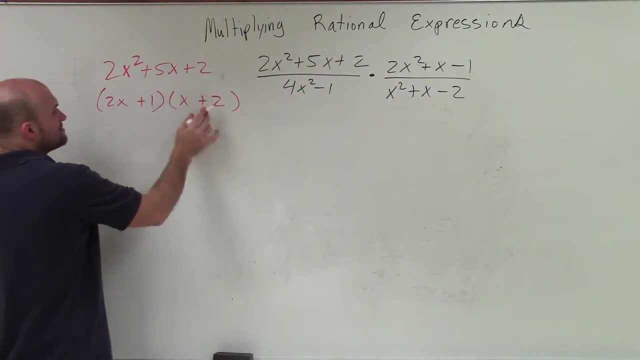 to add up to a positive 5.. So we can probably eliminate now our negative numbers and just use the positive. So what we need to say is: all right, what do I need to multiply 2 by and then multiply x by, so therefore they add us up to 5? Well, I realize that if I do 2x times 2, that gives. 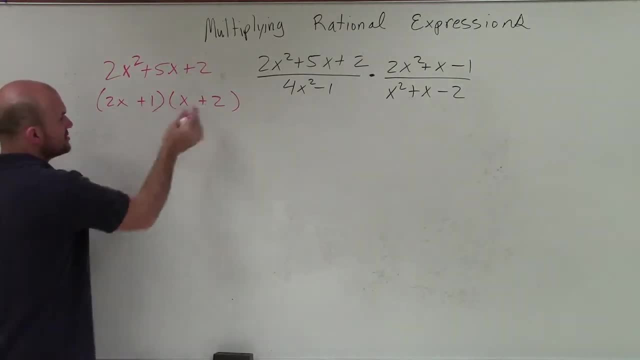 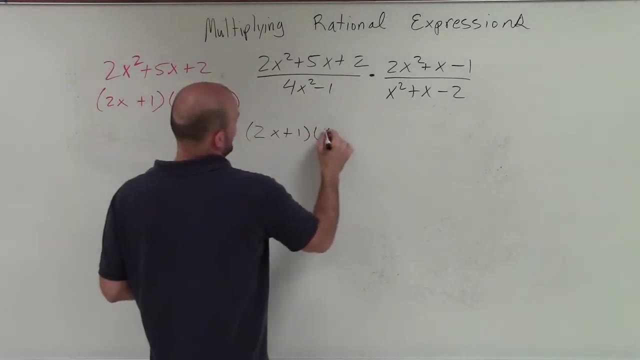 me 4x plus x times 1 gives me 5x. So therefore that's going to be my factored form for this trinomial. So I have 2x plus 1 times x plus 2.. Then over here I have a difference of. 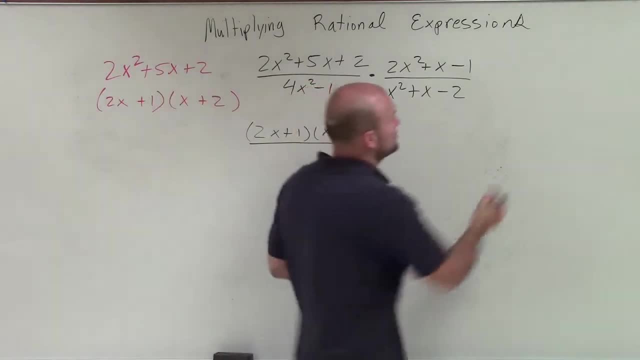 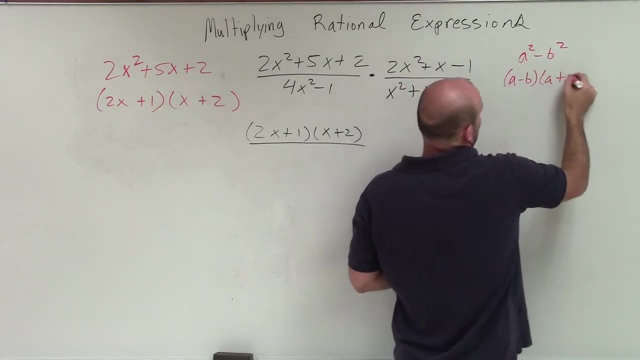 two squares. Now, believe it or not, remember difference of two squares. all difference of two squares states is if I have a squared minus b squared, that can be written as a minus b times a plus b, But you might say: all right, yeah, well, this one has a 4x squared though. Well is. 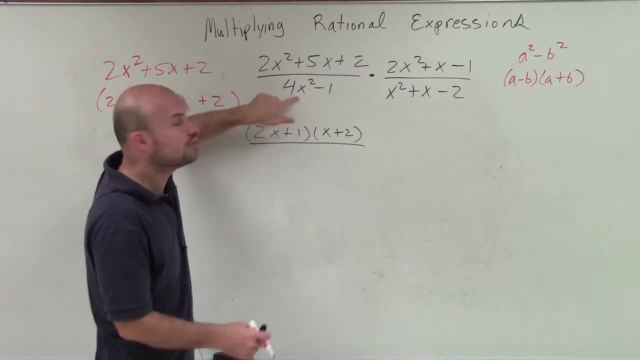 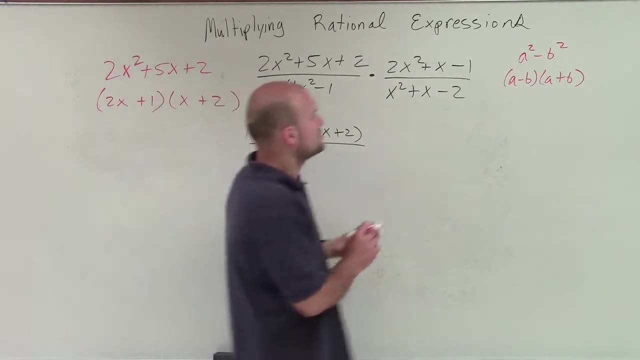 4 a square number? Yes. Is x a square number? Yes. So this whole term is a squared term that we can rewrite. And is 1 a squared number? Of course, 1 times 1 squared is 1.. So therefore, 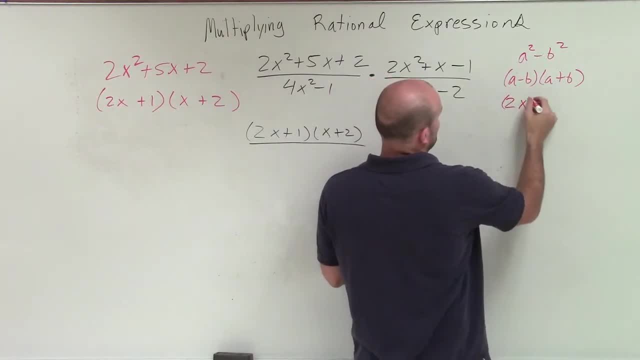 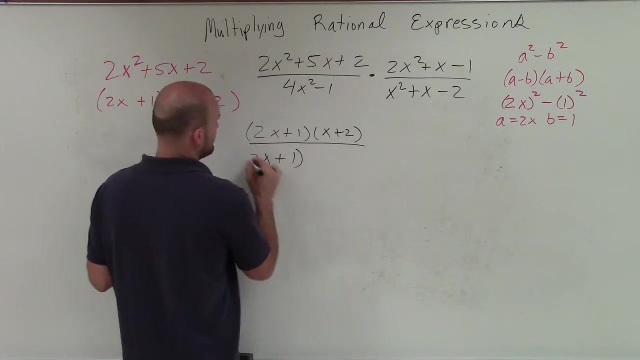 I could rewrite this as 2x squared, 2x squared minus 1, squared where a is equal to 2x and b is equal to 1.. So, therefore, the factored form of this is going to be 2x plus 1 times 2x minus 1.. All right, Pretty cool. 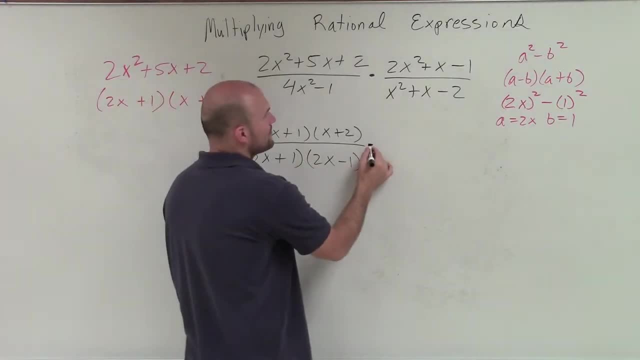 here, And then we already know we're going to be able to divide those out, But let's continue. So now I have 2x plus 1 minus 1.. And again, thankfully, we just have the 2 in front, So it's going to be pretty basic. 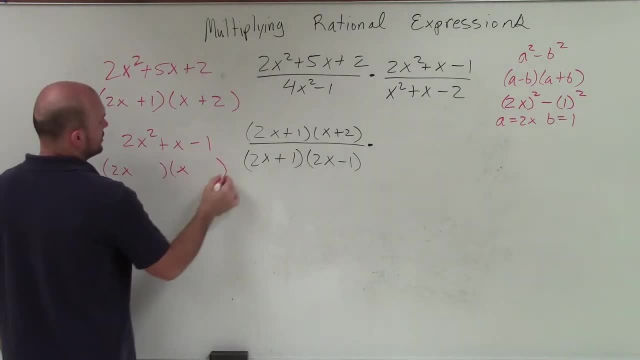 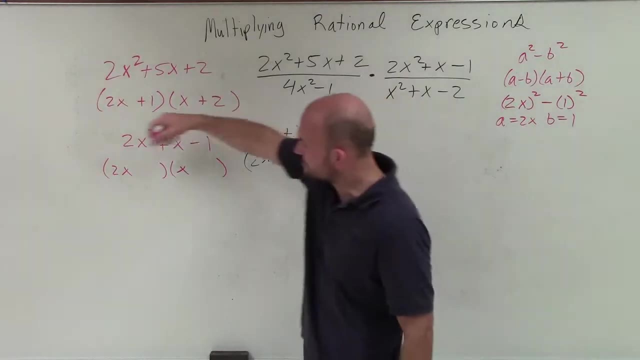 For us when determining our two factors. we know they're going to have to be 2x and x. And then I just know that now my last two terms- so we know the first two terms- have to give us 2x squared. The last two terms have to give us negative 1.. So it's either: 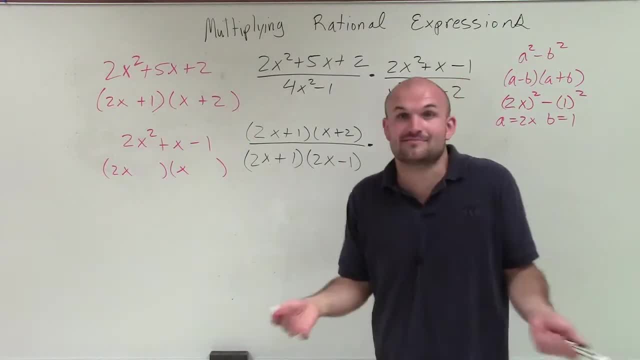 positive 1, negative 1, or negative 1, positive 1.. It doesn't matter, It's supposed to be both 1.. But 1 has to be positive, 1 has to be negative. Now we know my middle term has. 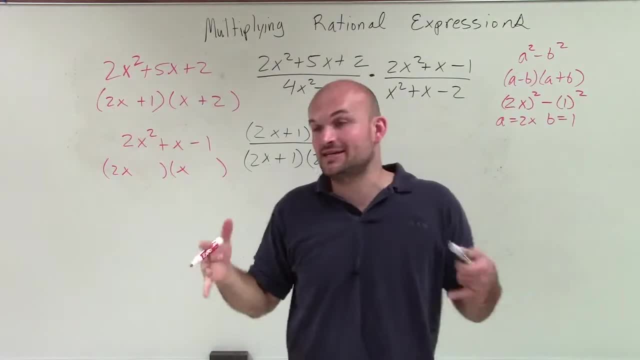 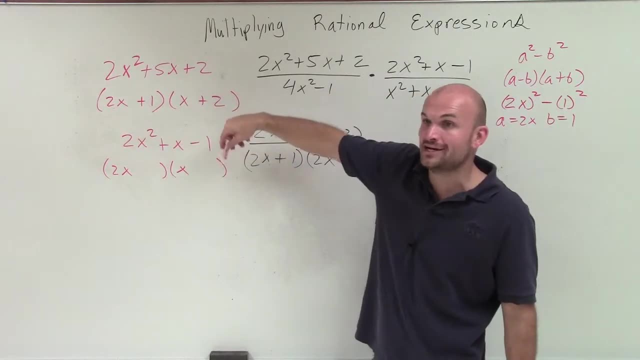 to add up to 1.. Therefore, the larger of my products, either in the outer or in the inner, is positive. Well, I know that if I multiply 2 times my outer 1, I know that has to be. that's going to be my larger product, because the inner would be just an x. So this has 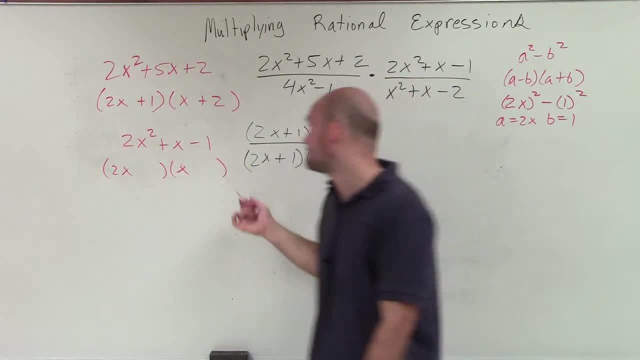 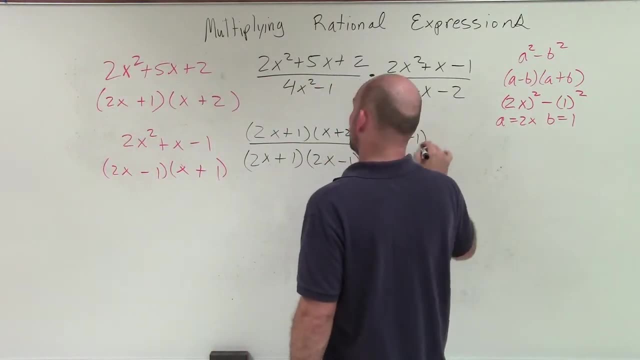 to be whatever I multiply the 2x by has to be positive, So that's going to be positive 1. And that will be minus 1.. So therefore, I rewrite that as 2x minus 1 times x plus 1.. All right, And I'll explain my thought again, Because, remember, we know that, that 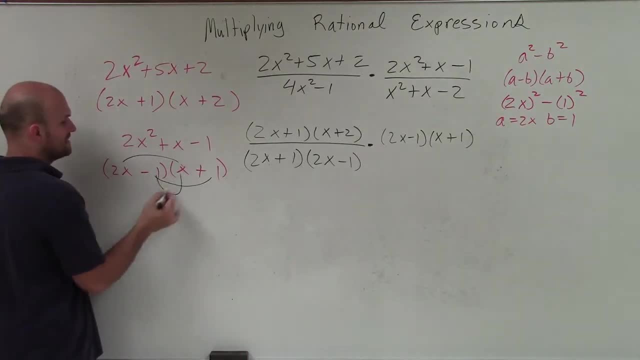 goes to 2x squared, We know that goes to negative 1.. Now the addition of my outer and my inner have to give me x. Well, 2x times 1 is positive, 2x Negative. 1 times x is negative x. So 2x minus x is 1x. All right Then, thankfully. 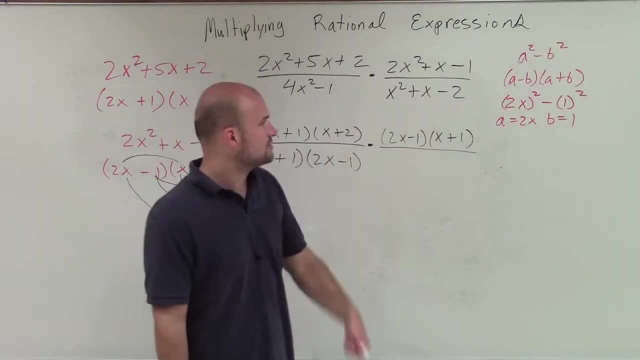 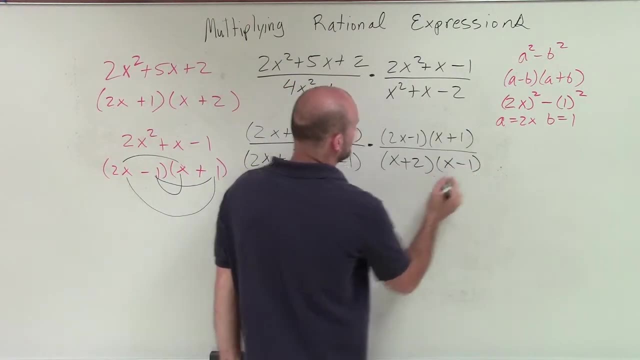 now we can just do a basic factor technique. What's two terms multiplied to give me negative 2, but then add to give me a positive 1? That's going to be x plus 2 times x minus 1.. All right, Now I know I have binomials that are separated by addition and subtraction. However, 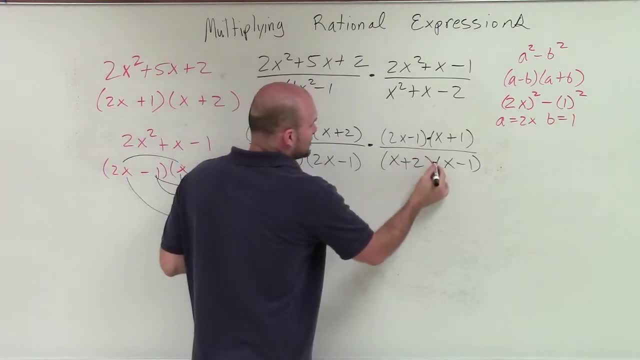 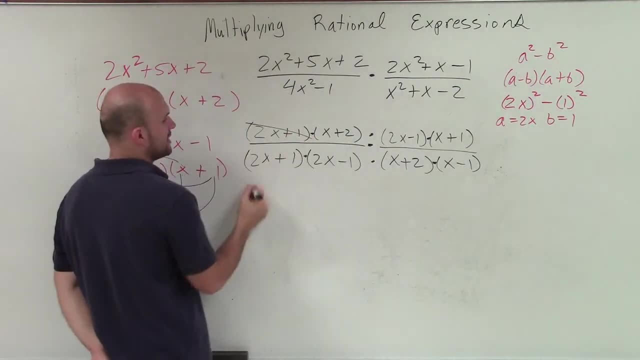 every single binomial, though, is separated by multiplication, So therefore I can divide across this multiplication. So now I'm just going to take whatever's in my numerator and in the denominator. If they're exactly the same, I know they divide out to 1.. So we don't. 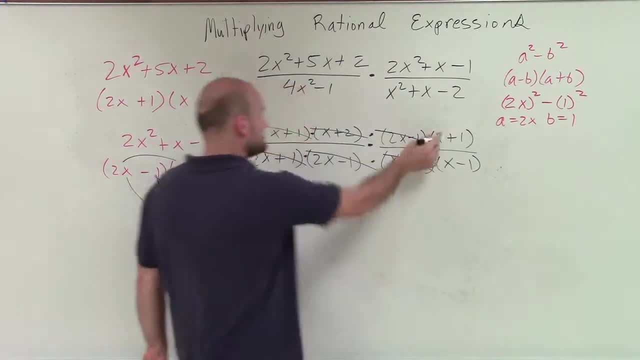 need to keep on including them, And these are close but not exactly the same. So, therefore, my final answer is going to be x plus 1 over x minus 1.. So there you go, ladies and gentlemen. That is how you multiply rational expressions. Thanks, Oh my god.